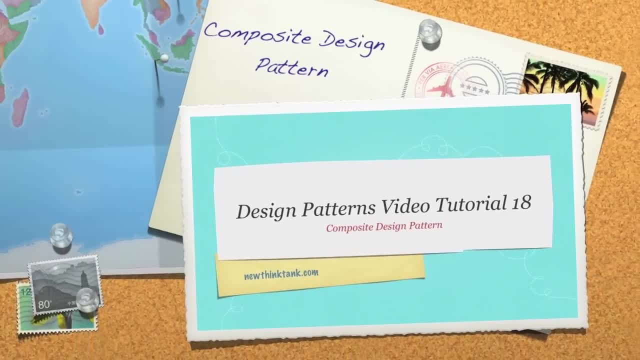 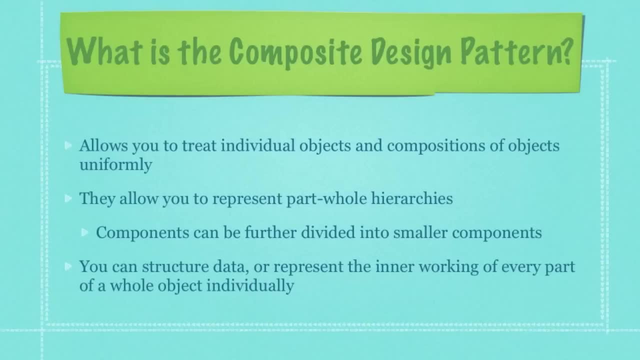 Well, hello internet, and welcome to part 18 of my design patterns video tutorial. Today we're going to talk about the composite design pattern. Now, the composite design pattern is another one of those two patterns that sounds really complicated whenever you read the definition of it, but once 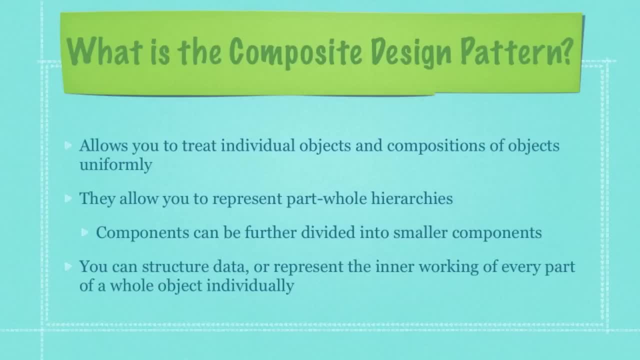 you see the code and you see it in pictures. it makes a hundred percent sense. So, either way, I'm going to go in and read the common definitions for it. It allows you to treat individual objects and compositions of objects uniformly. That is the typical definition for the composite design. 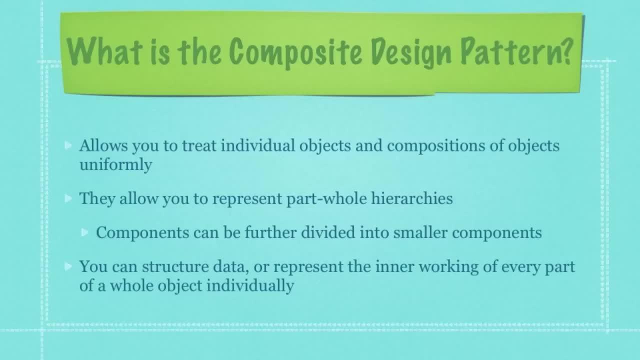 pattern, Then you have they allow you to represent part whole hierarchies. What a part whole hierarchy is simply is it's when components can further be divided into smaller and smaller components. And then a more logical definition is: the composite design pattern allows you to structure data or 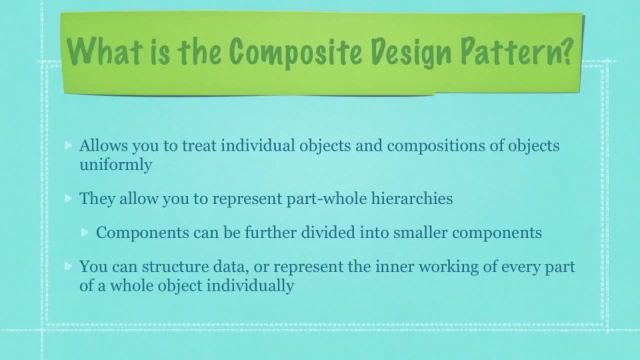 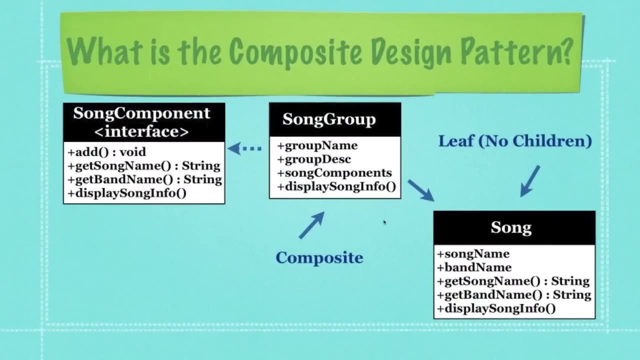 represent the inner working of every part of a whole object individually. If you didn't quite get that, let's look at some pictures. Okay, so in this demonstration I'm actually going to use exactly what you see here on the screen. First, you're gonna have your component. what this is going to be is an interface that's going to be inherited by the composite, and what? 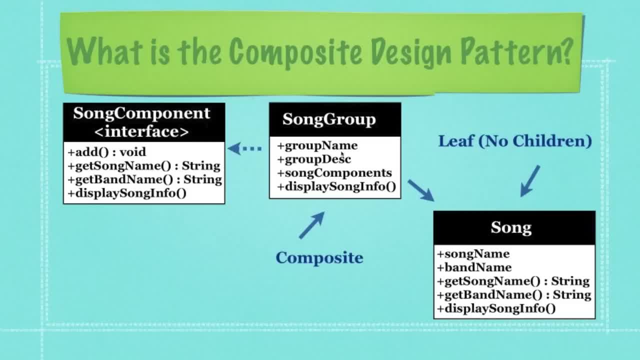 the composite is going to hold in this situation are either going to be groups of songs or individual songs, And then you have your individual songs, which are going to be called leafs. Difference between a composite is a composite can contain once again songs or groups of songs. Here's a 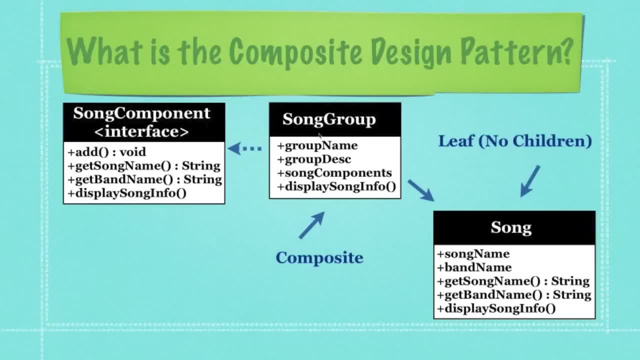 song, and here's a group of songs, so a composite can actually contain composites, while a song or leaf has no children objects at all, Then what we're going to be doing here is, in this interface, we're going to define exactly what we have here. 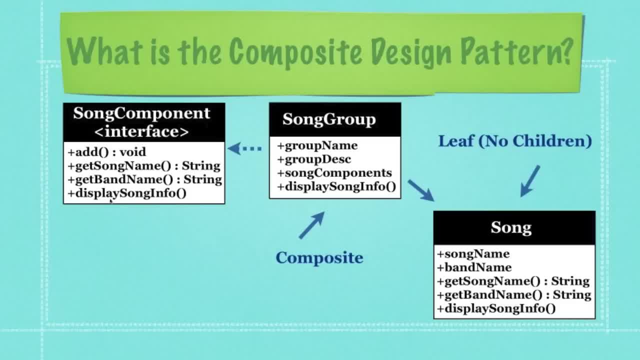 meaning we're going to be able to define song names, band names and then display that information That's going to be inherited by the group here or the composite, and each group is going to have a name and a description and it's going to be full. 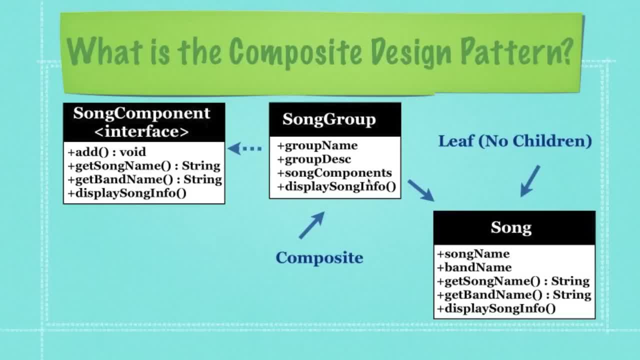 of, in this situation, an array list of songs that we're going to call song components. It's also going to be able to display information in regards to both the song group as well as the individual songs. Then you're going to have your songs, you're going to have a song name. 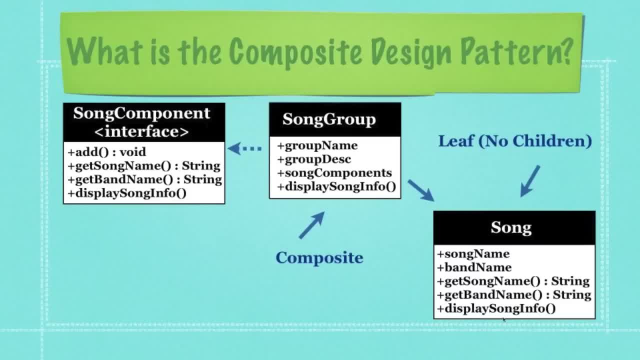 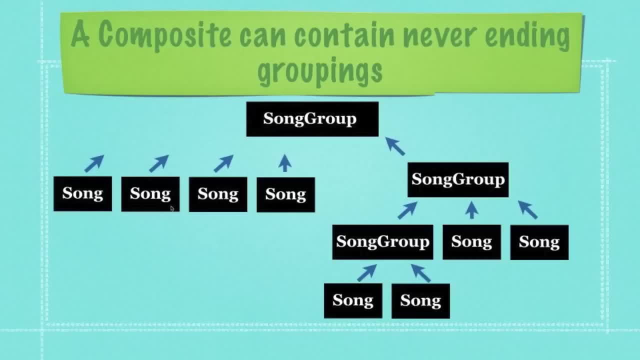 band name, you're going to be able to exactly get a hold of those and also once again display all those. To look at this in a more logical way, here is a song group, which can either be made up of just songs or a song group that contains other song groups. 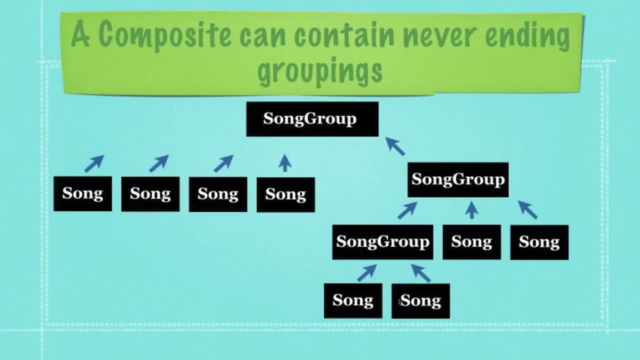 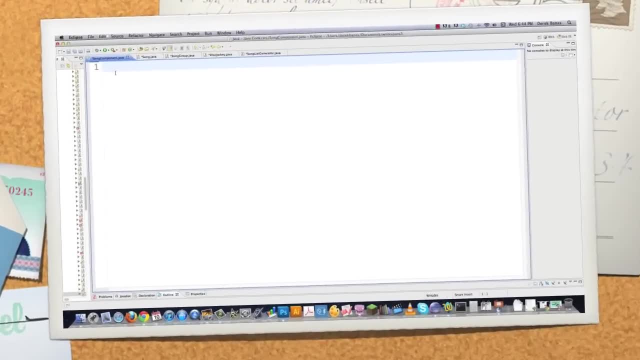 including songs, or just songs, just like you have right here. So that's an overview of the composite design pattern. so let's get started, Let's get into the code and make it a hundred percent understandable. So here we are in Eclipse, and the first thing we're going to do is we're going to create: 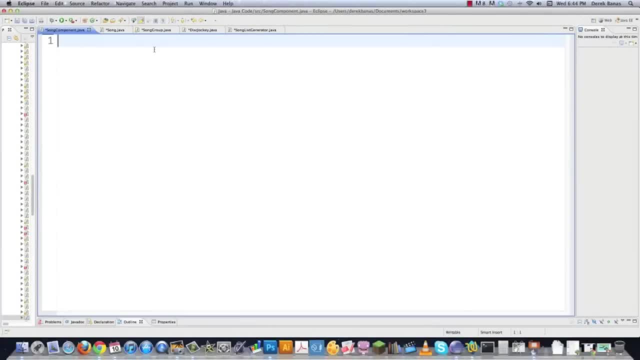 song component dot java. This is the component using the jargon, and what we're going to do is create an abstract class and of course, we're going to call it song component, and then we're going to define everything that we could ever use inside of this, Of course, spell. 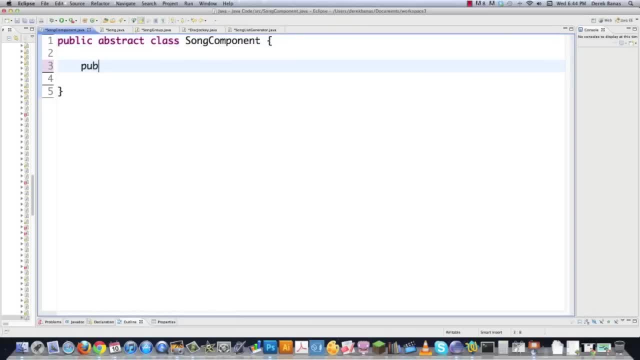 abstract, right Alright. so we're going to just jump right in and we're going to define some things here That I'm actually not going to use inside the tutorial, just to give you an overview of the type of things you could do. So let's say we wanted to be able to. 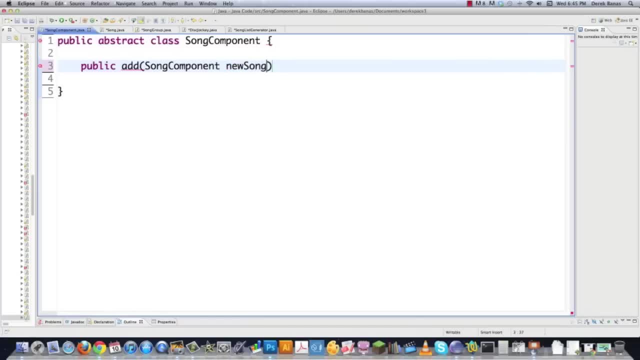 add song components. We're just going to go: new song component and then, quite simply, what we're going to do here is we're going to throw an exception- unsupported operation exception- which is a very common exception that you haven't seen until this point. Basically, what this guy is saying here is that we're going to throw the unsupported 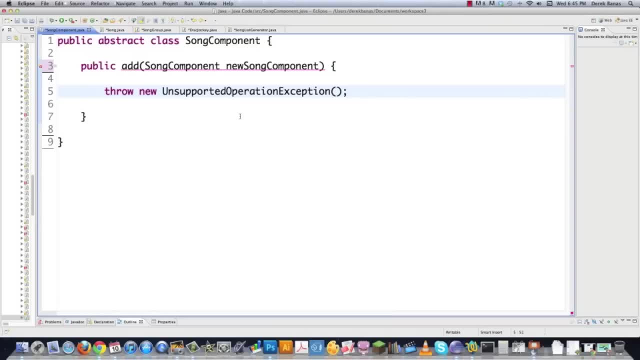 operation exception: if it doesn't make sense for a song or song group to inherit a method, and in those situations in which it doesn't make sense, they're just going to inherit the default implementation. You don't need to worry too much about what that means. We're going to get more into that at a 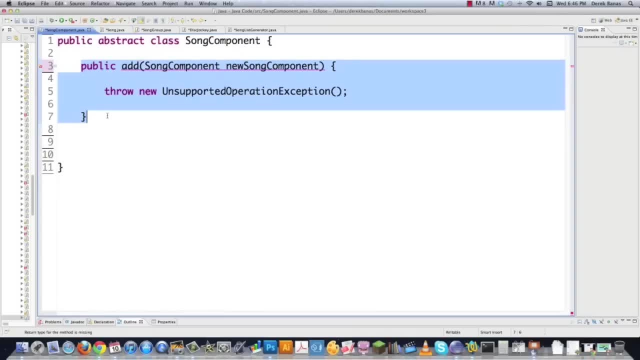 later date, Then another thing we're going to have to do is, if we can add components, we may also need to remove components. Basically, what we're doing here is just defining all the different types of methods that we may need in the future, and I'm going to throw a void. 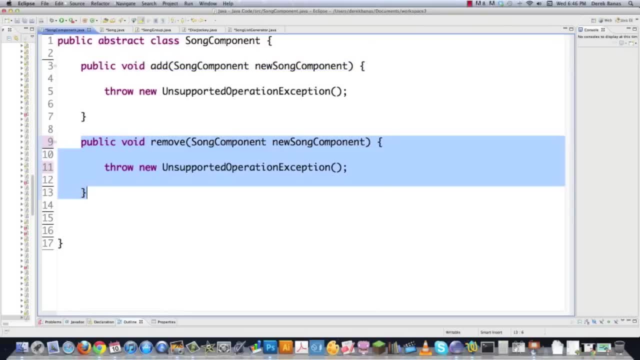 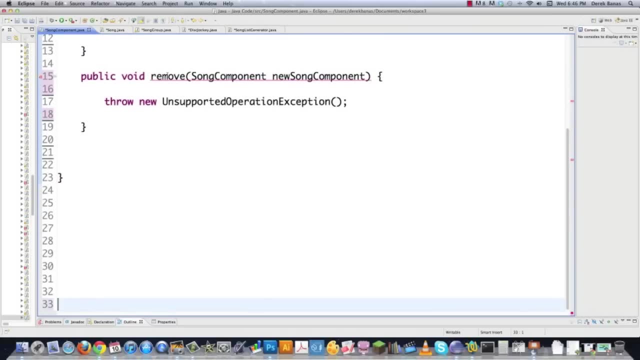 inside of there and void inside of here as well. Another thing you might want to do here is get a component, and a component, like I said before, is going to be groups of songs as well as individual songs, which we're going to define here in a second. 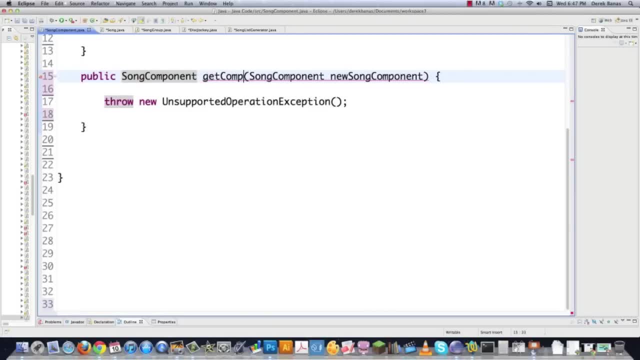 Song component. We might also want to be able to get our components, and you can say something like component index- Let's actually spell that out- And then something we are going to use is get name, and this is of course, going to be a string, and then 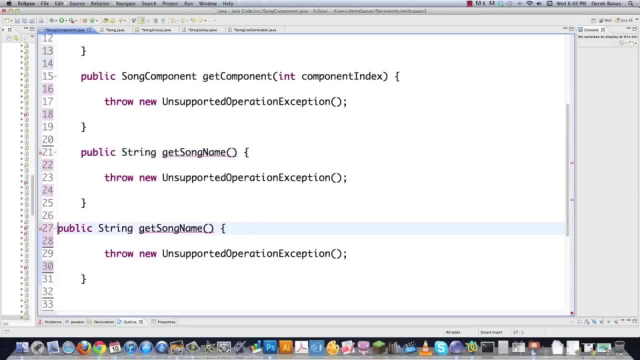 to require any attributes be sent to it and then get band names, since we're going to be playing around with song names and band names and we could also, like we did in the previous part of this tutorial, return the release year for this song. basically, what we're doing is kind of like we did. 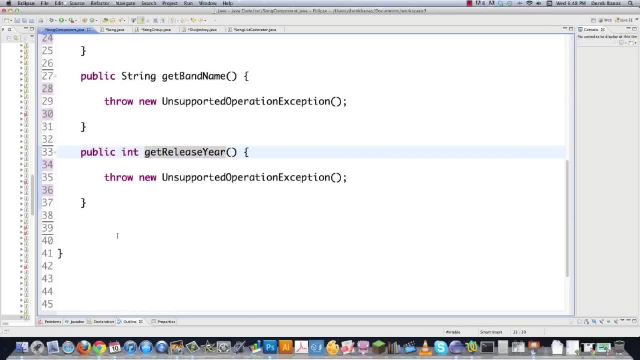 with the iterator design pattern, we're going to be creating tools for a disc jockey to be able to pull information out in regards to songs. and then this final one here is very important because this is going to be used to display song information as well as groups of song information, and we're 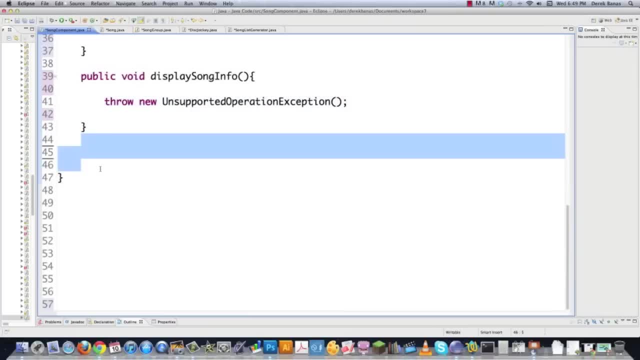 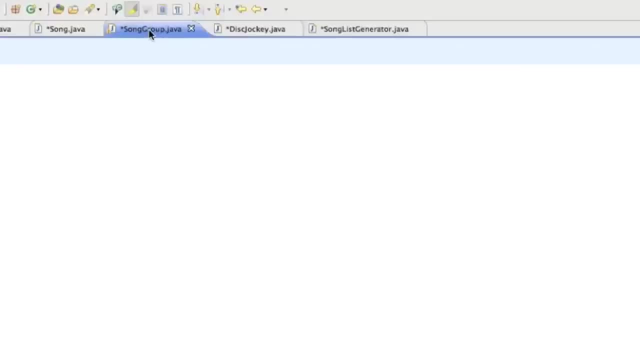 also going to throw that exception right there, basically just defining all the things that might be used in everything that is going to extend this abstract class. so now let's jump over into songgroupjava and start defining some groupings where we're going to be saving this information. 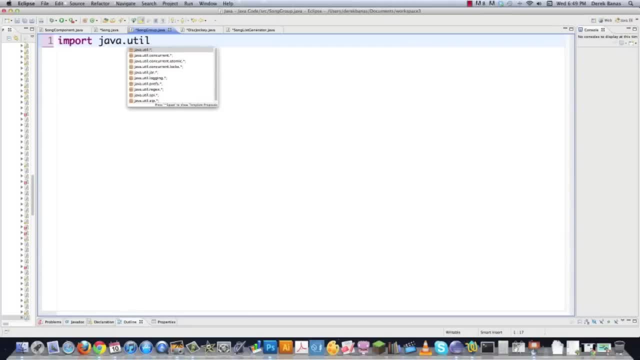 and i'm going to be using an array list because, i said before, all these songs are going to be stored in this array list and i'm going to be saving this information in this array list, an array list- and I'm going to cycle through songs using the iterator that we 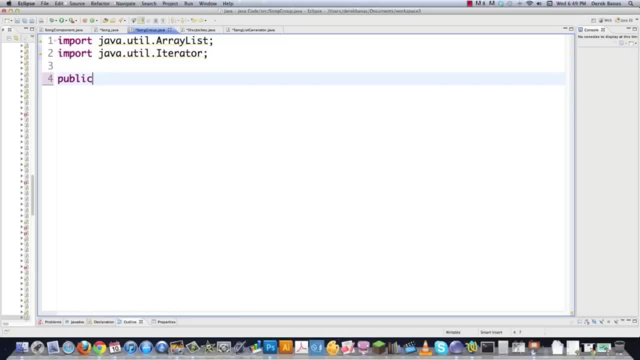 talked about in the last part of this tutorial, and then we're going to go public class- song group extends song component, which we just created a second ago, and then we're going to create our array list, which is going to contain any songs or song groups are going to be added to any of the other songs or song. 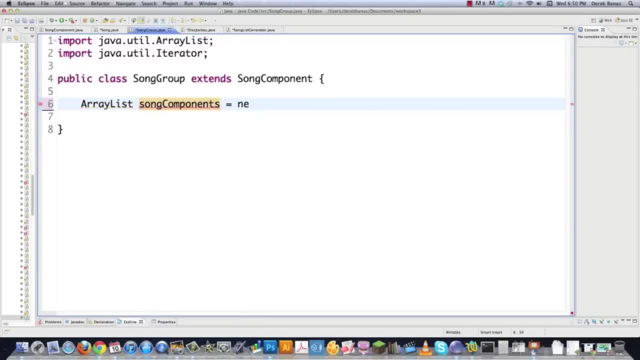 groups and I'm going to call this song. components is equal to new array list and all of this code can be had underneath of this video. click on the link and you can get it, and it's heavily commented to help you understand everything. so we're gonna have group name and another thing is gonna be group. 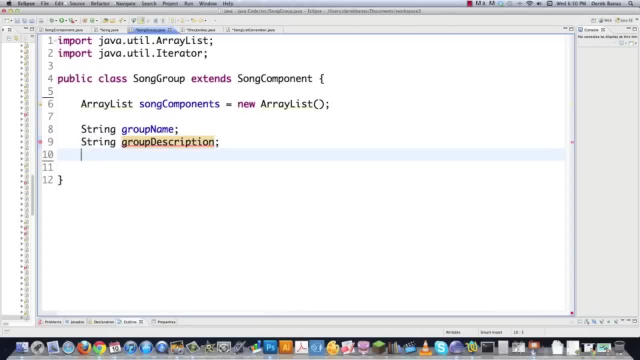 description, because what I'm basically going to do is put some different forms of music, provide a description of those different forms of music, like heavy metal, and then a description of heavy metal, and then I'm gonna have them a whole bunch of songs that are heavy metal songs inside of it. so this is sort 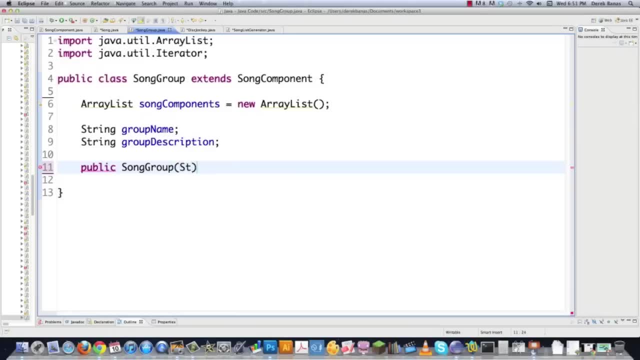 of using the composite pattern to describe data, but you could use it to describe pretty much anything and it's going to be passed a group name and a group description and that's it. I'm gonna change this to new group description. then I'm just gonna be able to go group. 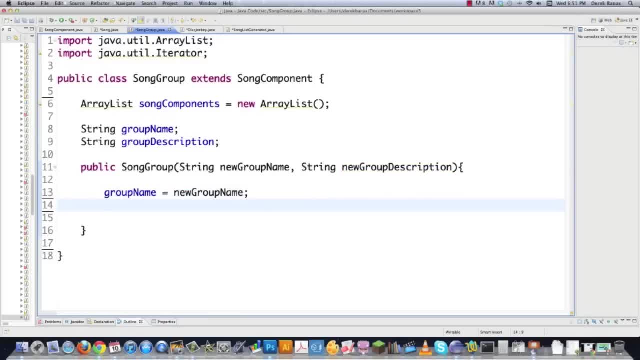 name is equal to new group name and group description is equal to new group description. okay, so that's just going to set up those defaults, pretty simple stuff. then we need to provide access to the group name and the group description, and it's just going to be a little bit more complicated, but I'm just going to 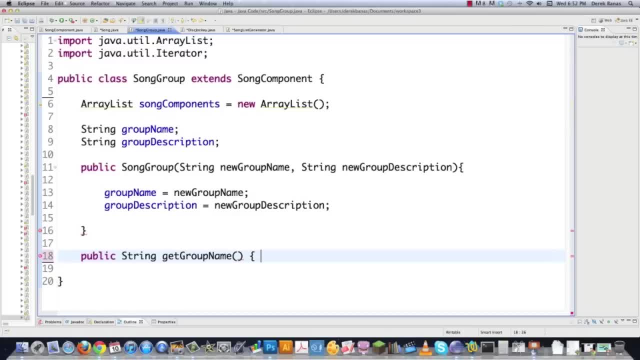 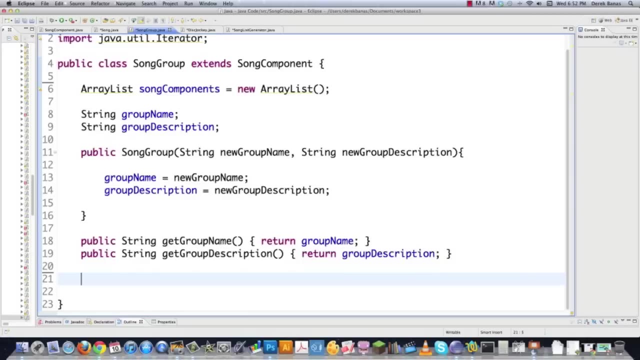 be: get group name real simple. I'm gonna keep this all on one line, right, like that, and then I'm gonna copy this and provide an easy way to get group description, like that, and this is going to be group description. so very simple stuff so far. like I said, this isn't a very complicated pattern to understand. 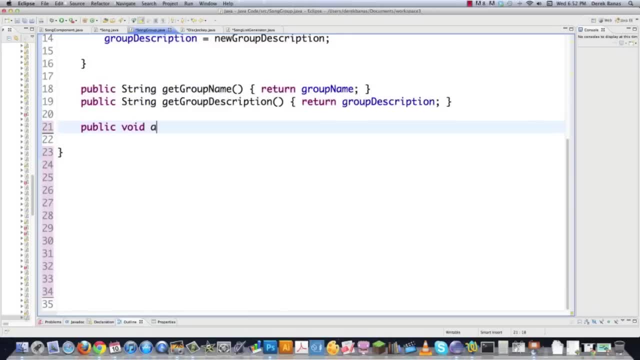 then we're gonna need a way for them to be able to add either groups of songs or individual songs to this. so we're gonna add the individual song components and then to actually add to them, I'm gonna go song components and add them to that array list that we created above. like that pretty simple and even though 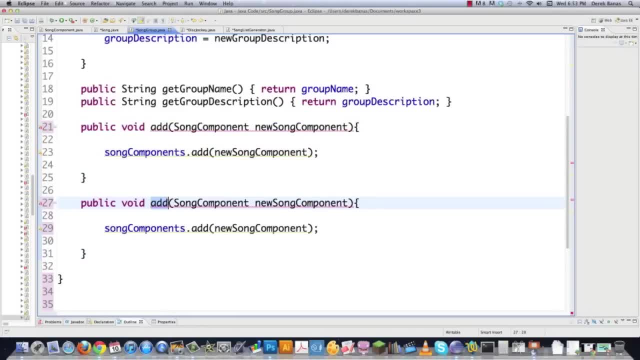 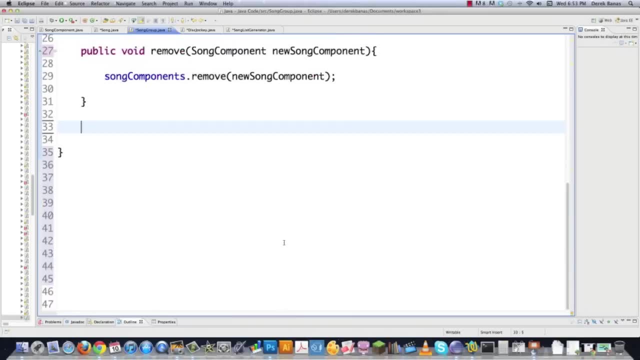 I'm not going to get into it in this part of the tutorial. I'm gonna allow you to remove individual song components. real simple, just go remove instead of add. pretty simple. these are just gonna make changes to our array list. and then, of course, we're going to provide song component the option to get song. 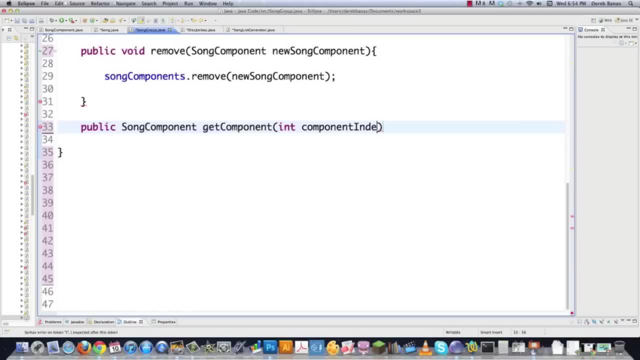 components and that's gonna be int component index. in the array we're gonna have to cast this to be a song component, like that: song components, which is just my array list again, and I'm gonna get the right one by passing at the index. so there we are, pretty simple stuff, and then this is slightly complicated. but 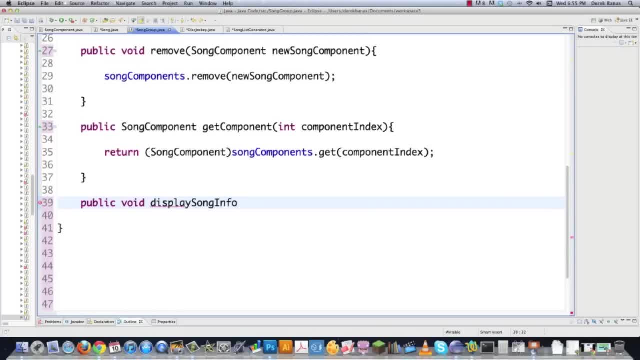 not really. we're gonna go display song info, just like we created previously in the interface that we extended here, and I'm gonna go system out print line, say get group name. put a space inside of there. like I said, group name is gonna be something like heavy metal and then afterwards we're going to list a whole. 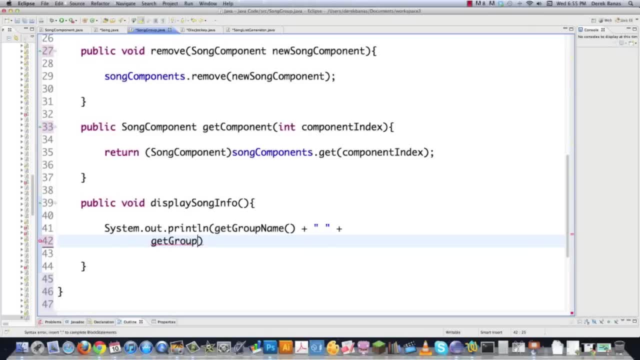 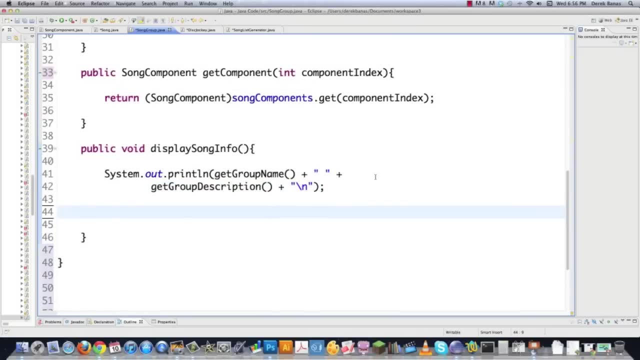 bunch of heavy metal bands, but first we're going to provide a description of what heavy metal is and then throw a new line in there. alright, so if I'm gonna be able to, or if I plan on printing on a list of songs, well, how do I do that? I'm 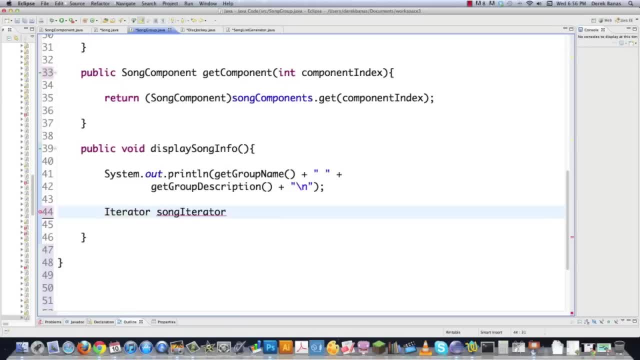 gonna use the iterator trick that we did in the previous video. I'm gonna use the iterator trick that we did in the previous iterator design pattern tutorial and since everything's a component or a song component, gonna be very easy for me to change everything into an iterator. there you are: just changed everything into an iterator and 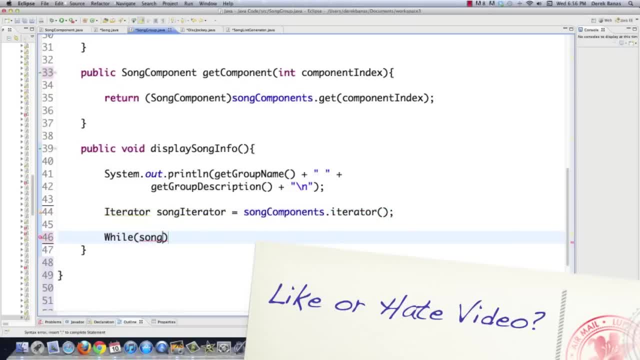 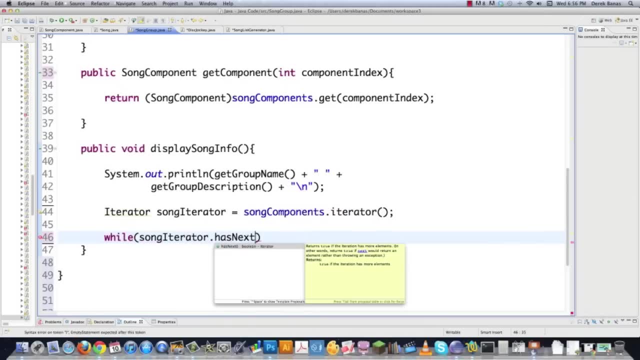 now that I have that iterator created, that's gonna allow me to iterate through all of the songs and song groupings that are inside of each song group. song iterator call has next like that: I'm gonna go song component: song info. we're gonna do a cast, just like we did. 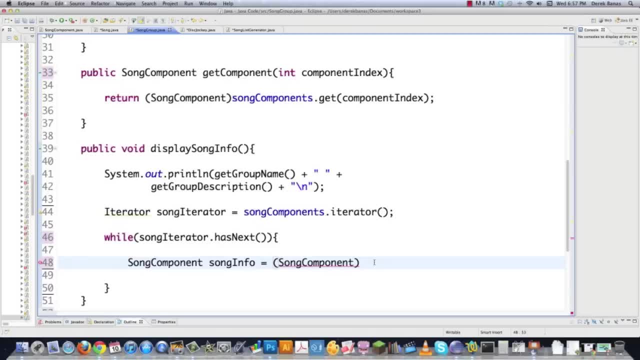 up here. I'm gonna cast what's in the array list into a single song component and we'll go song iterator and ask for the next one in there. and then we're gonna go song info and call display song info so that it displays the information on the individual song. and now that we did all that for all those songs, what we 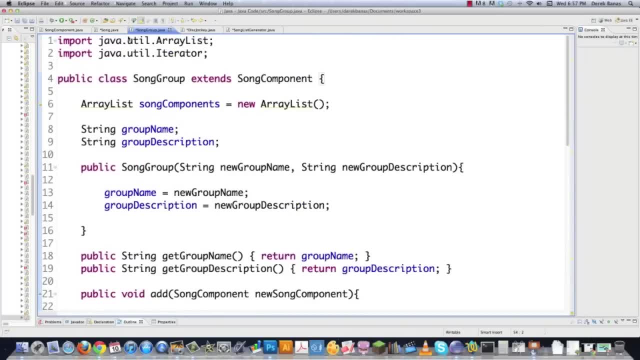 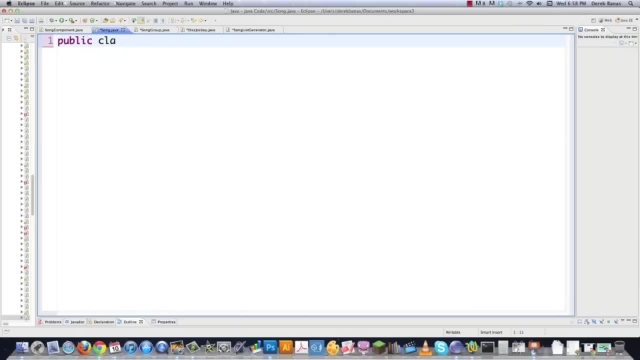 need to do now is go and actually create song dot Java, which is right here. this is just gonna be information in regards to the individual song. So I'm going to go class song. I'm going to also extend song component so that I'll be able to treat the songs and the song groupings the same to take advantage of. 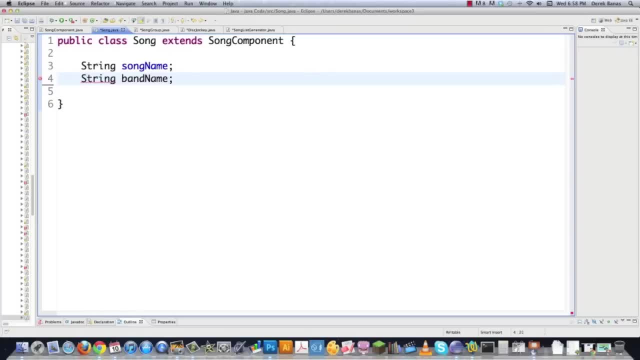 polymorphism. Now I'm going to go band name and int release year, like that. And then what do we need to do? Go public, allow them to provide us information on the song. So they're going to pass us new song name, the new song they want to add to our little tool we're creating here. And then 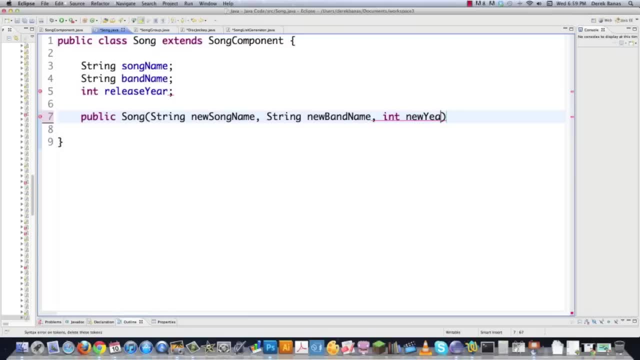 we got a new band name And then they're also going to give us year release. All of that information is going to be passed in and we're going to use that information to create a new song object. So just go: song song name: new song name, band name: new band name, release year: new release year There. 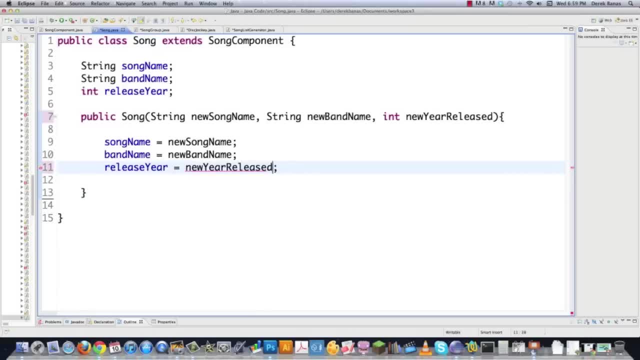 you are. Now you can create song objects. So go like that and put a D there. Now we're ready to go And we're very close to being done. We're going to go public string, get song name, and now we're. 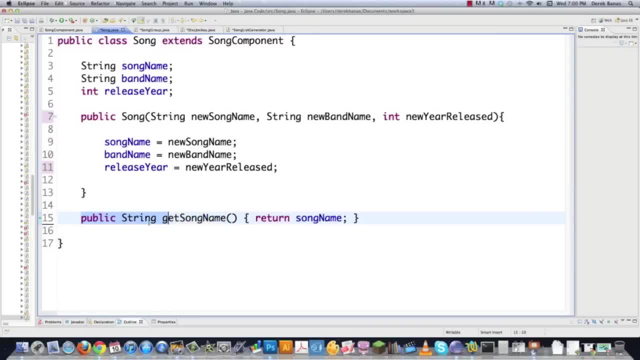 going to. We'll be able to return our song name, of course, And then we're also going to have to provide access to band name and release year And, of course, make that an integer. All right, pretty simple Now all. 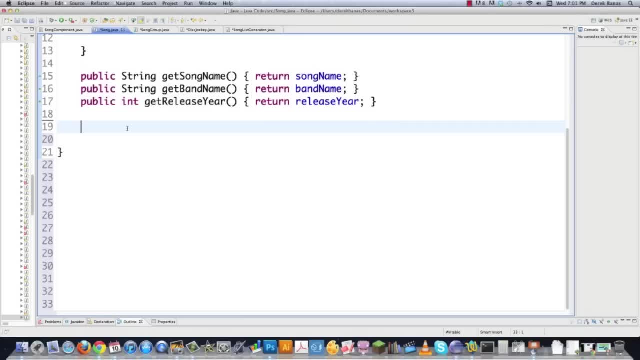 we need to do is provide the ability to print out all of that song information that we just got. And what are we going to do? We're going to go public void, just like we did with song component right here display song info. So I might as well just copy this guy, jump back over into songjava. 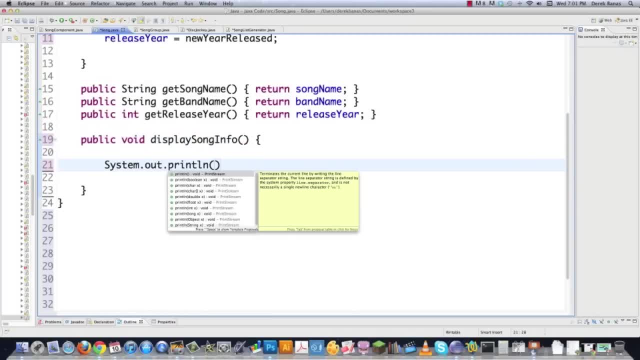 public void: doink. there it is. system out Print line: get song name was recorded by and then get band name And then we'll say something like in get release year. So that's going to print out all the information that we need in regards to. 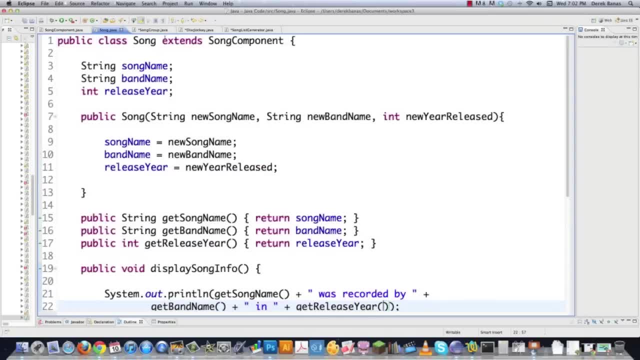 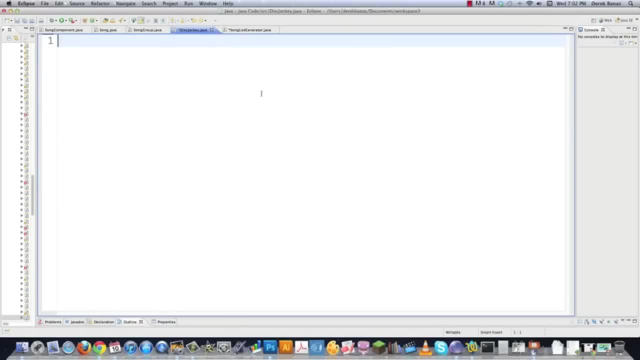 our individual songs. So let's save it. And now we can go back into our disc jockey. Let's save song group. We're done with that. So discjockeyjava- you saw it in the last tutorial- We're going to. 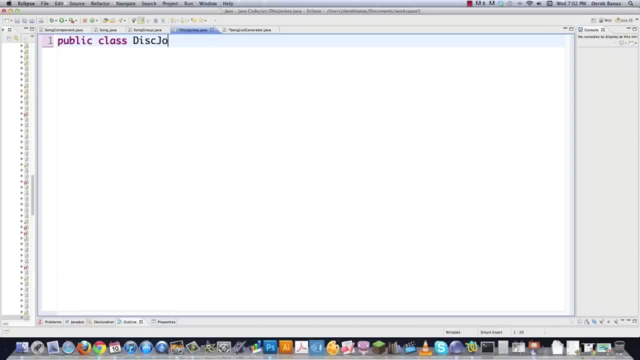 make it much easier to use. this time We're going to go public class disc jockey and this guy's going to feed up the songs and the groups of songs. So we're going to go public void, just like we did with the songs. We're going to create song component, song list and then public disc jockey. 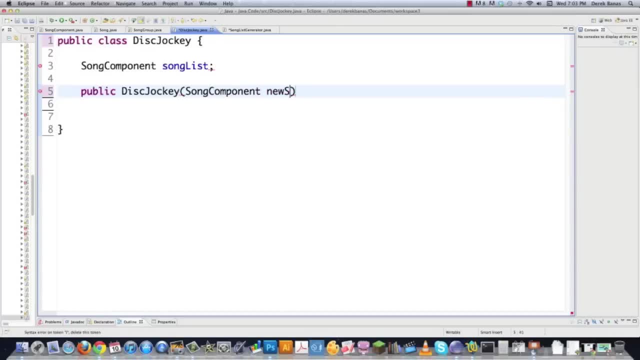 And it's going to be past a song component, new song list, And then it's just simply going to go: okay, well, my song list needs to be equal to the new song list that's just been passed to it. Piece of cake did that, And then we need to create another guy inside of here. that's going to 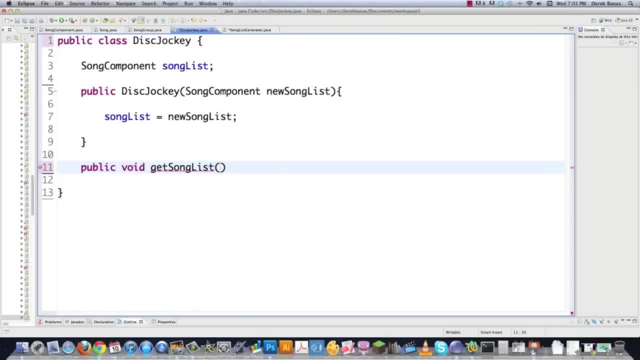 call all of the methods that are going to allow us to print out information in regards to the songs and song groupings. So we're going to go to song list display song info, which you've seen in every single object that extends song componentjava right up there. So save that. And now. 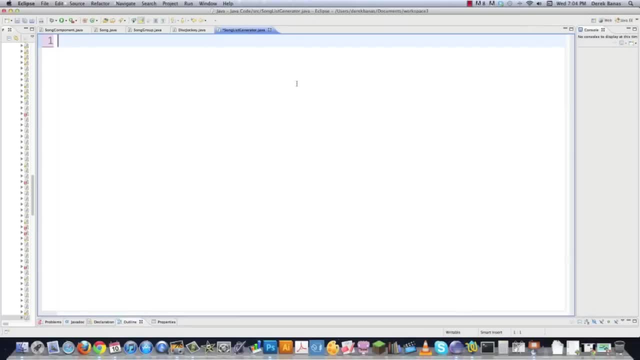 we need to go into song list generatorjava and make everything work, which is going to be really cool. So let's go. public class song list generator. public static void main. Now, inside of this song component, the first thing I'm going to do is create a song group, So I'm going to go to the 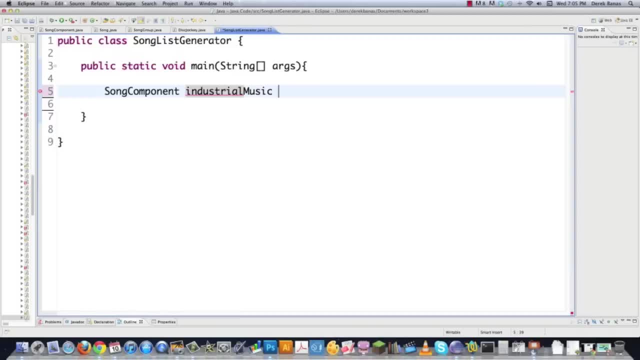 a song grouping. So I'm going to go. industrial music is going to be the name of it. You can think of this like a folder that's going to contain a whole bunch of industrial bands And in fact it's also going to contain another song grouping, And then there's going to be a 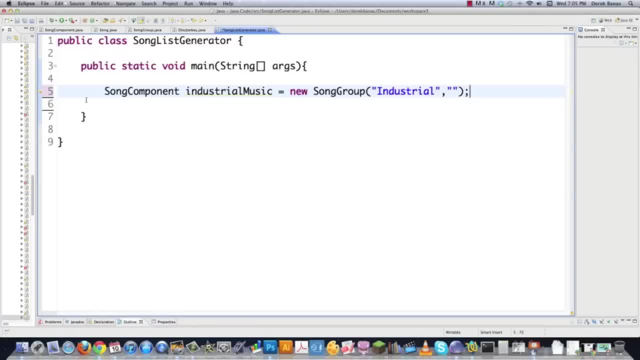 description inside of there, which I'm going to leave out for a second because I'm going to copy and paste that to save myself from typing something ridiculous that doesn't really even matter. And then the next one I'm going to create here is heavy metal music, And this is just going to be. 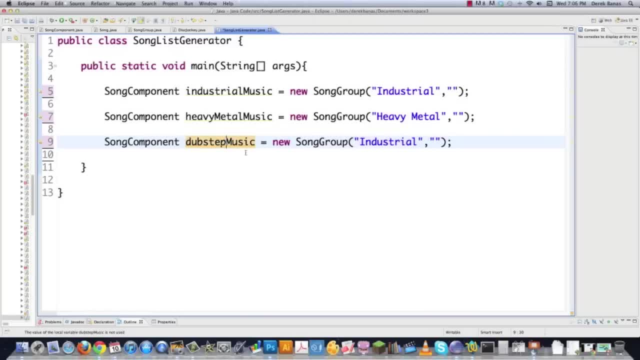 heavy metal, And then what seems to be very popular now, dubstep. Don't murder me on this. I'm going to consider dubstep a version of industrial music. So dubstep is actually going to be inside of a song group, that is, inside of the song group called industrial music or the. 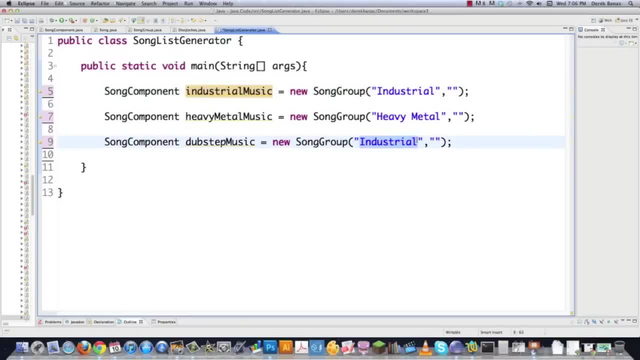 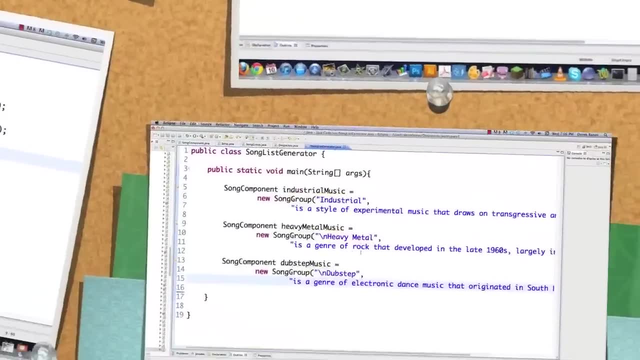 folder. Every time I say song group, you can just think folder whatever you want to think. Jargon wise, that is definitely wrong. But what are you going to do? I'm going to copy and paste all this additional information in here. Okay, so there's industrial music, heavy metal music and dubstep. 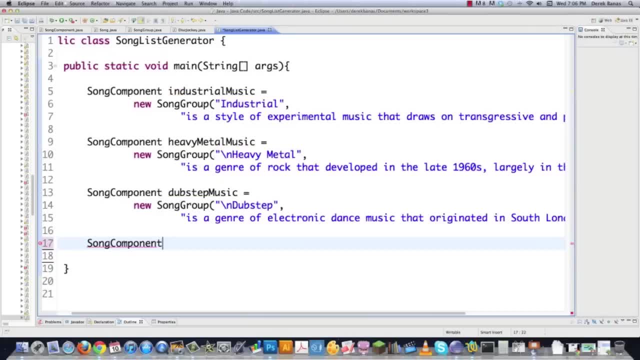 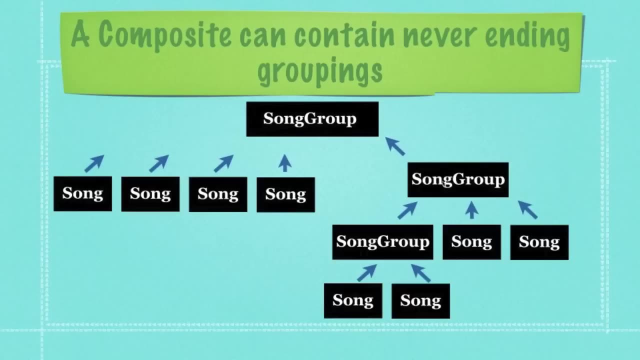 with a description For each one of those. then I need to create a top level component that's going to hold every single song group and every single individual song, every song. This is all I'm doing here. See, this is the song group. That's what I'm creating right now. There's individual songs. This is the song group. 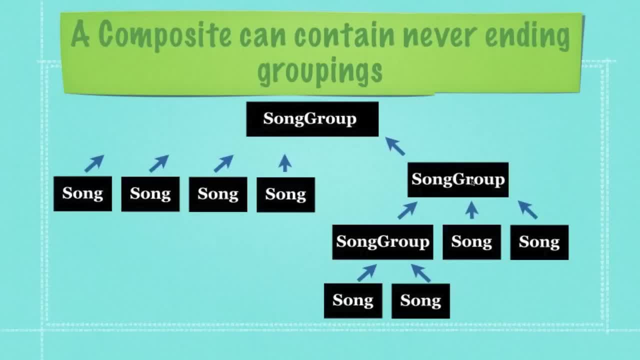 These are going to be industrial and heavy metal and dubstep and all that, And then it's going to be in the situation with industrial music. This song group is going to be dubstep and it's going to have songs inside of it. So that's what's going on here. I'm making right now in 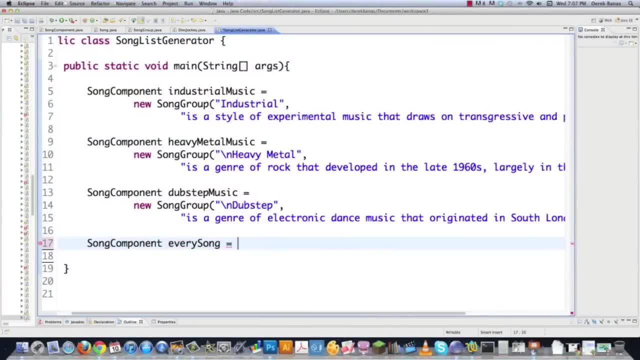 code what you see on the screen. Okay, so here's every song which is the master song grouping. So to do that I'm going to go new song group- See, it's the same. And I'm going to call that song list because every song 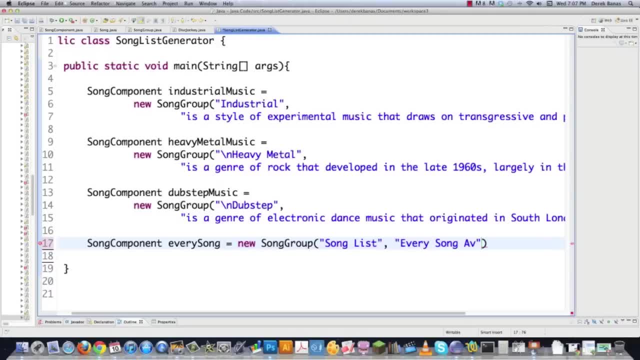 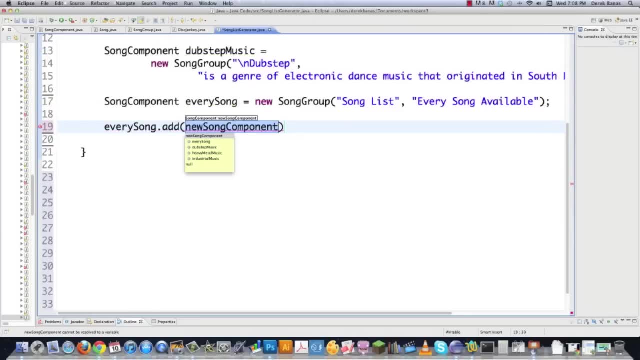 group needs a title and it also needs a description, because we said it did That's going to hold everything. Then I'm going to go every song and I'm going to add my groupings inside of it. So what's one of the groupings that we said we're going to have inside of it? Well, industrial music is going. 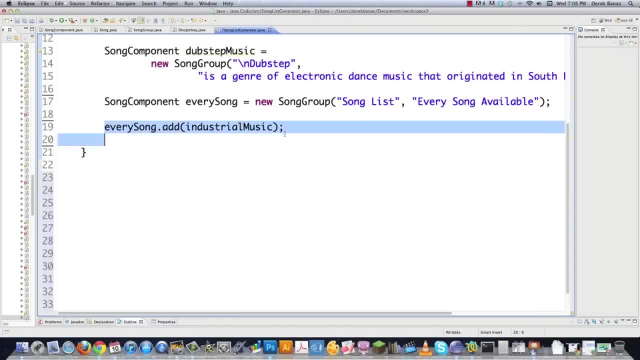 to be one of them. And there you are. I just added industrial music, which is a folder inside of the master folder, And now if I want to add an individual song into industrial music, I just need to go industrial music, add new song. 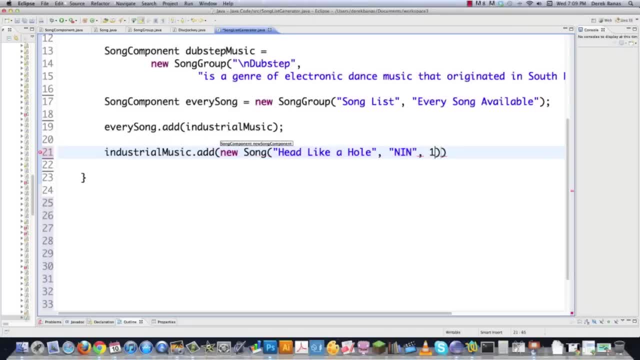 and then make a title for a song and a band name and the year the song was released, And there you are All set. And then there's another band that's considered an industrial band, And then what do I need to do if I want to add an additional song grouping? 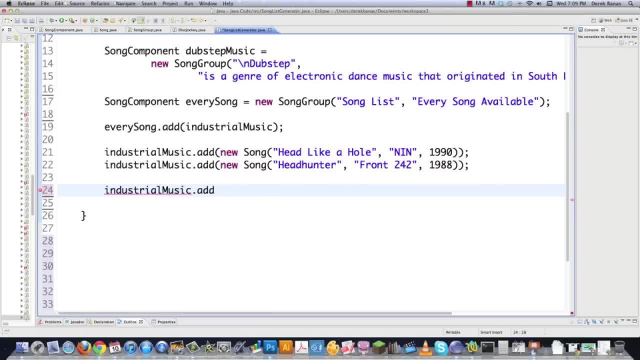 Inside of industrial music. I just go: industrial music, add, like that. And then let's say, I want to put dubstep inside of it. There you are. Now I can put songs inside of the dubstep music, music grouping or song group, which is exactly what I just did there. And then, of course, if I just wanted, 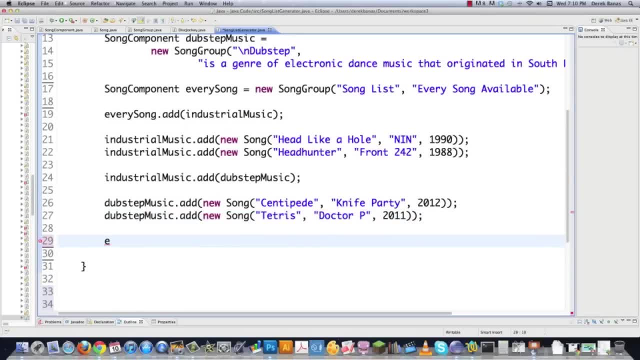 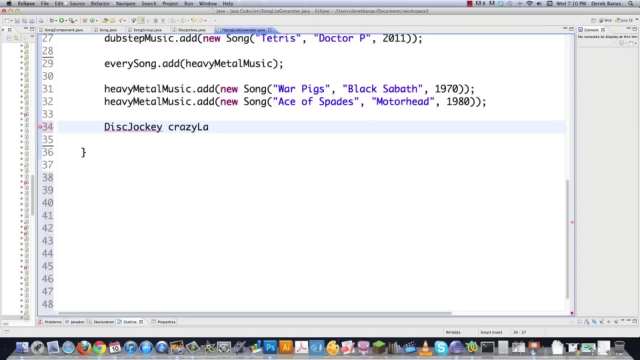 to have a song grouping that is going to have songs in it. well, that's very simple. Let's do that with heavy metal, Paste that there. So instead we're going to say heavy metal music And then, on top of- And now I'm going to call my disc jockey class that I created, I'm going to name my disc jockey. 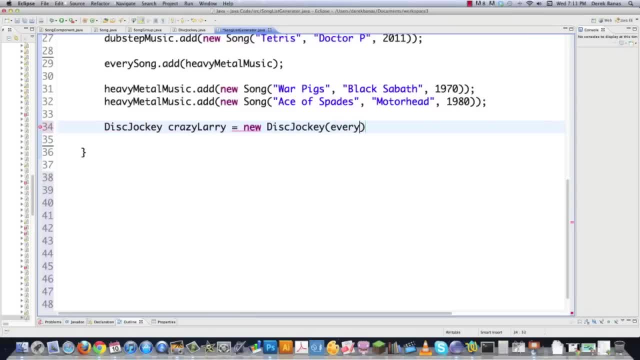 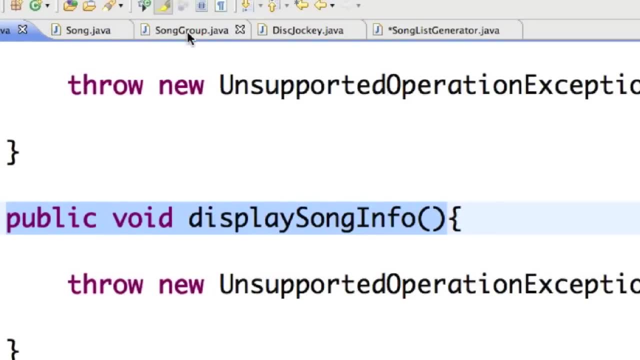 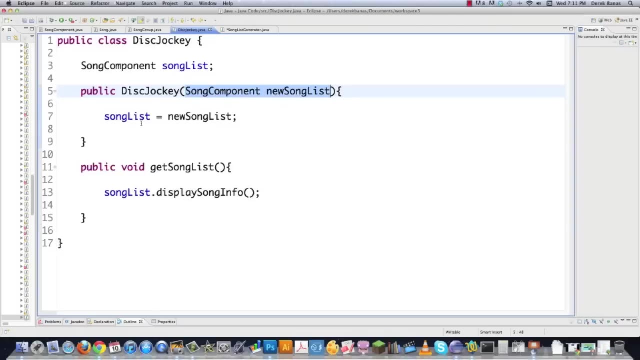 Crazy Larry, New disc jockey And I'm going to pass him every song which is of type song component, which everything is Song. Java and song group are both song components And as you see, here with disc jockey, here it is New song list And that is going to allow me to iterate through and print. 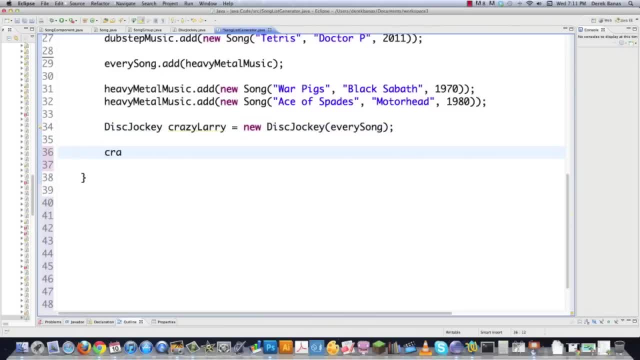 out. all that information Makes for some really tight code. Print it. I just go Crazy, Larry, Get song list Like that And like that And if we file, save it and execute you can see it cycled through it. Print it out First song list: Every song available: Industrial.